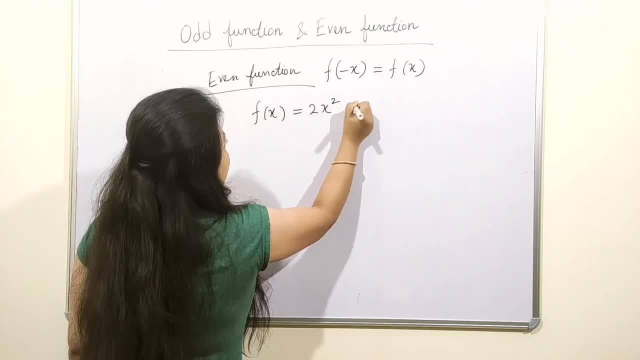 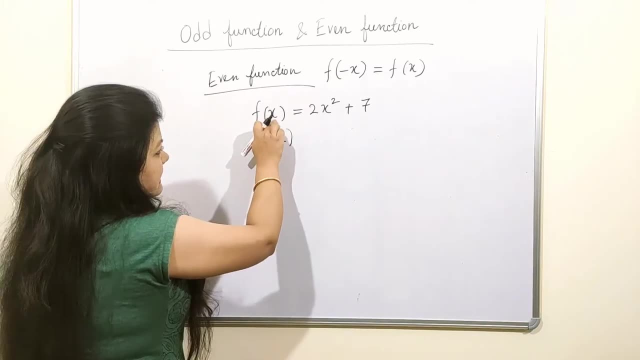 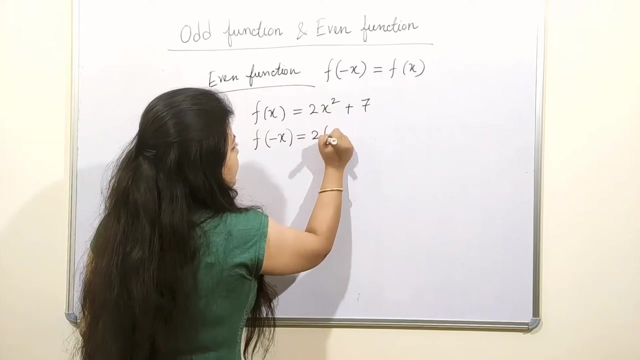 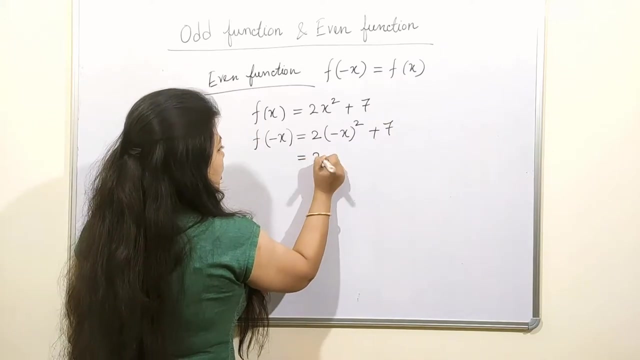 Suppose fx equal to 2x square plus 7.. Now here, what will we do In front of fx? we will replace divided by x. So by replacing this, value of x will be minus x and other values are same. So all of we know that. 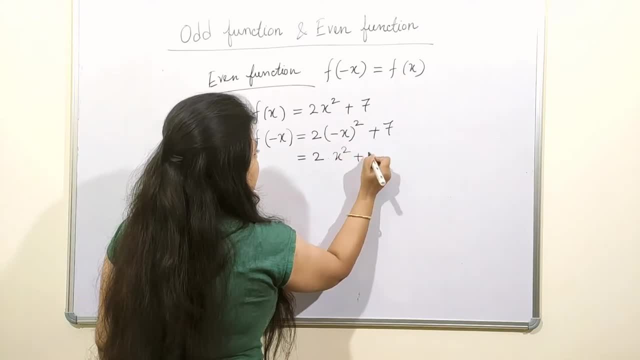 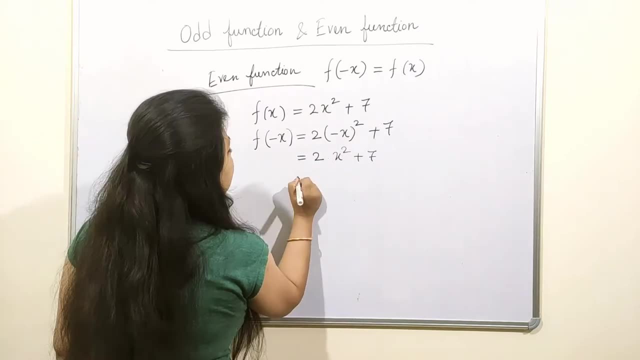 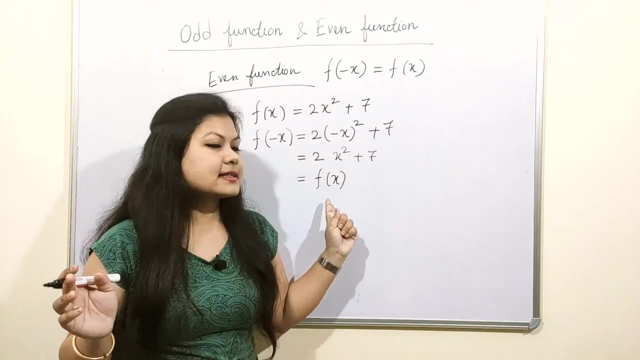 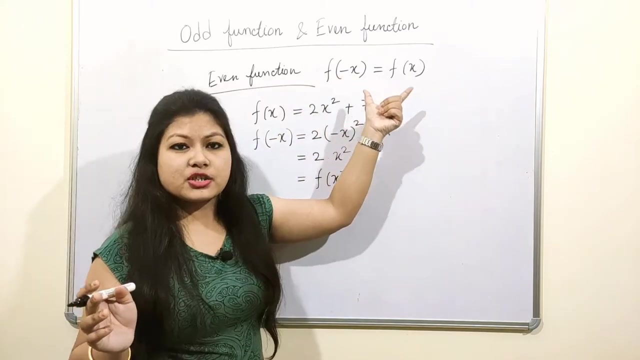 minus x square means it is also x square. Now you can see that we are getting the same value: 2x square plus 7. That means here we are getting the same fx value. That means f minus x, equal to fx. So what does this mean, This definition and this condition? 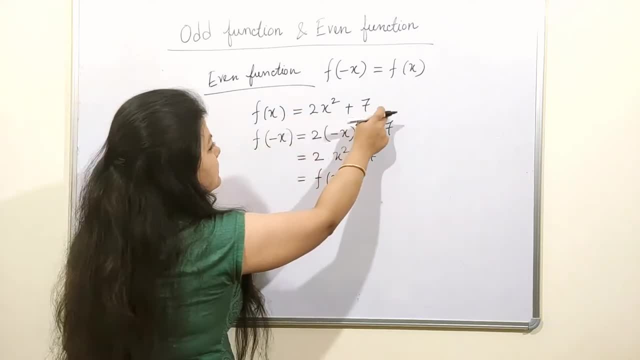 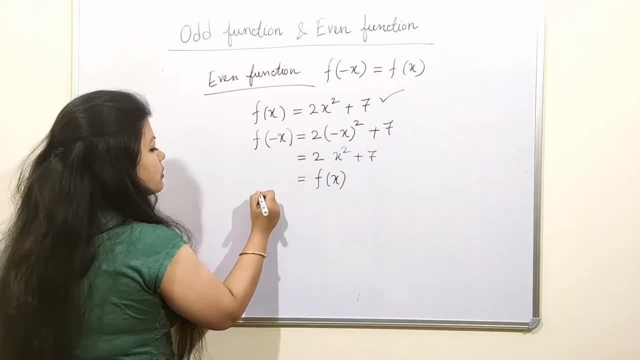 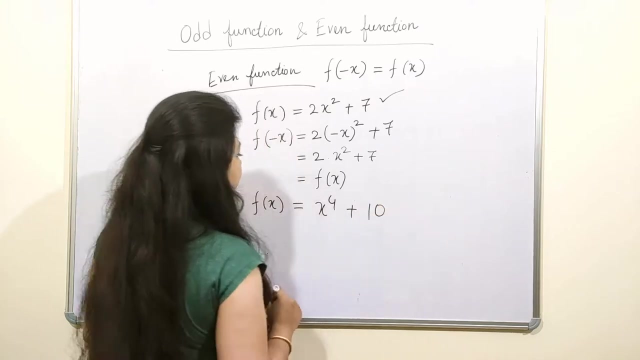 are being satisfied by this function. That's why this function will be called even function. And suppose we are getting this example x to the power 4 plus 10.. Now what will we do in this? Again, we will replace f minus x. 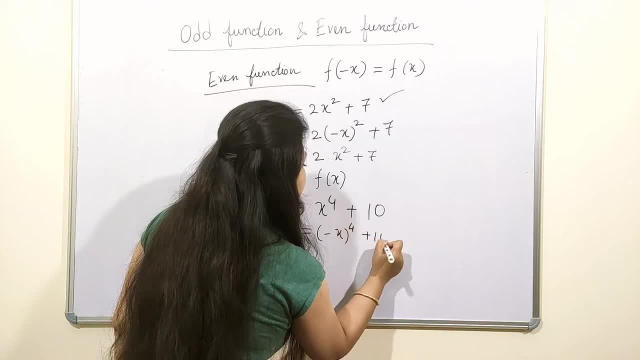 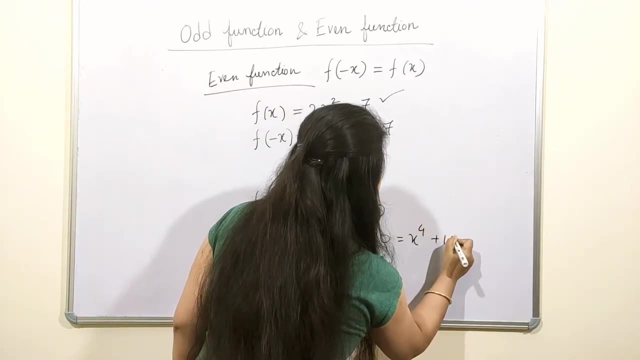 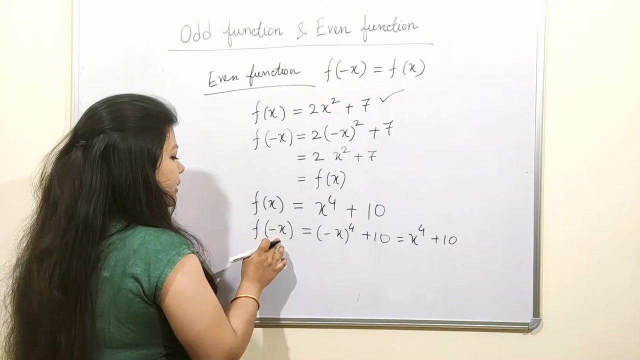 So it is minus x to the power 4 plus 10.. And we know that minus x to the power 4 is also x to the power 4.. So we again get the same function, function x to the power 4 plus 10. that's why, kya hua, f minus x, ka value equal to fx. so 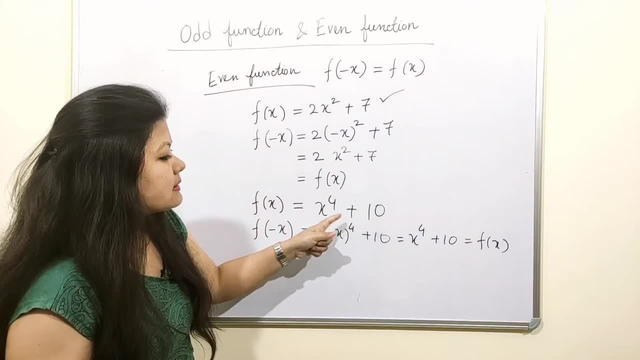 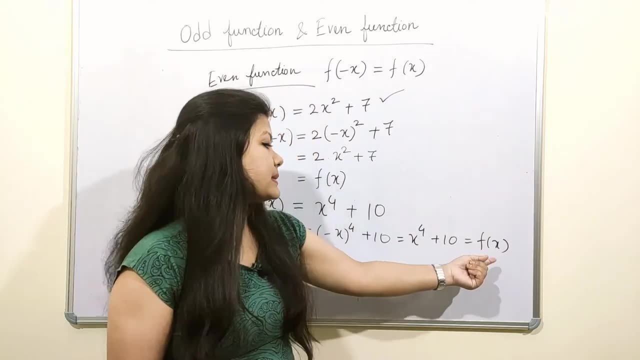 firse kya hua? x to the power 4 plus 10, this value ka bhi, agar minus x kesar hamro replace karte hai, fir bhi same value milta hai. that means, fx milta hai. that's why this type of 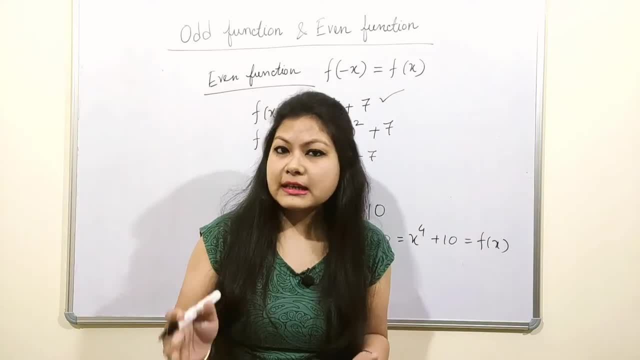 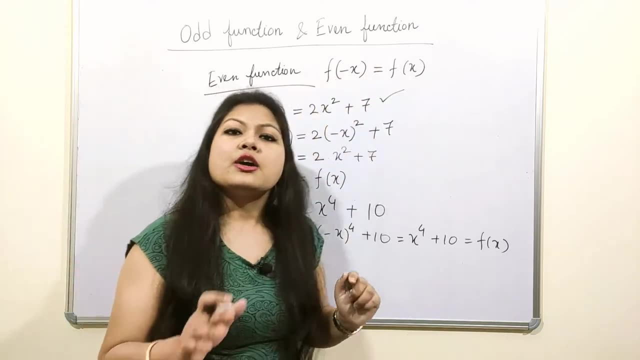 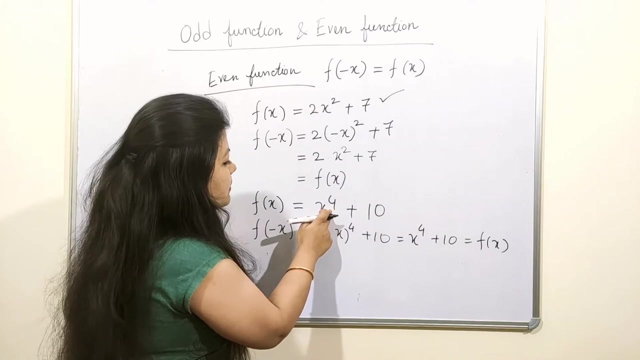 function is called event function. so basically, tumlogo ko kya yaag rakna hai this condition: whenever a function is satisfied by f minus x equal to fx, koi bhi function ho sakta hai. lekin basically ye yaag rakna ki jab bhi function x square, x to the power 4 or x to the power, 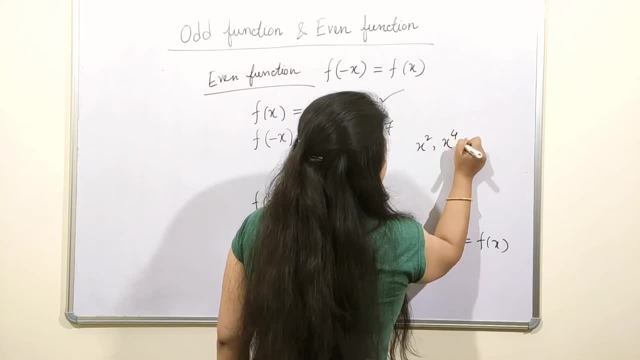 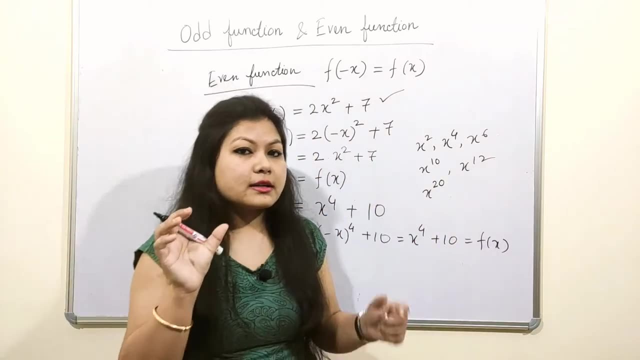 6, jese x square. x to the power 4, x to the power 6, x to the power 10, x to the power 12, x to the power 20 is type ka hamlogo ko. agar koi bhi value milta hai, toh bo function event. 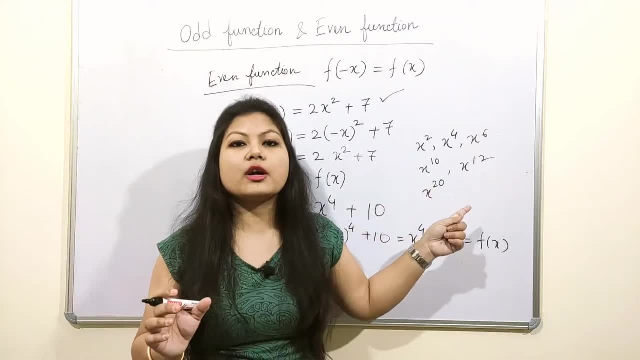 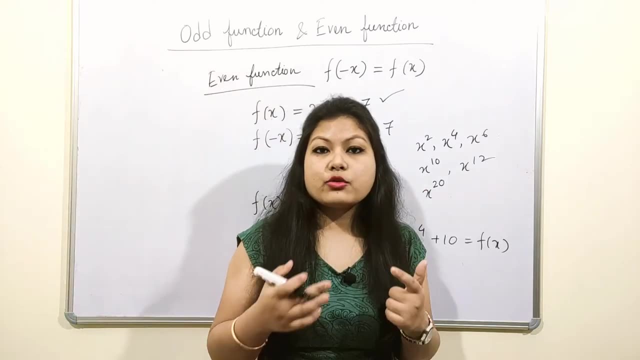 function hoga. so matlab ye yaag rakna ki x ke power jo hoga na ho. agar event number hoga na, toh ye hamesa event function hi hoga. lekin koi koi log kya karta hai koi koi student definition me ye? 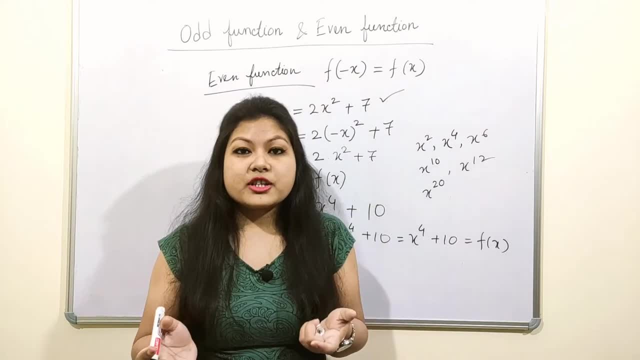 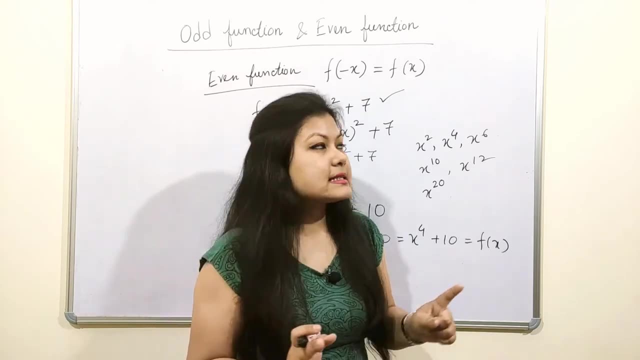 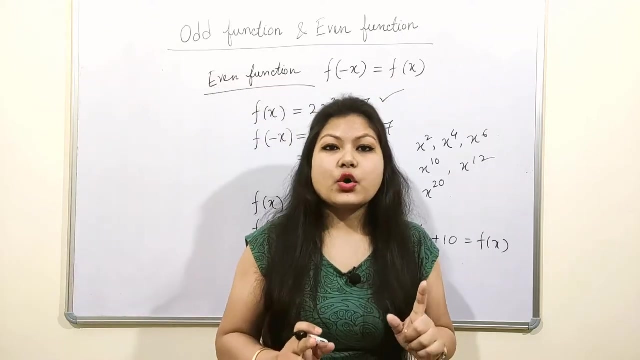 galti karta hai ki wo likta hai ki agar function me event value hai, then usko event function bolta hai. no, that is not the correct definition. correct definition is that whenever a function is satisfied by this condition- f minus x equal to fx- then it is called event function. 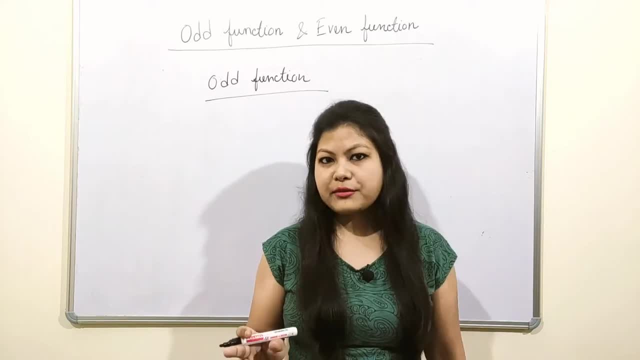 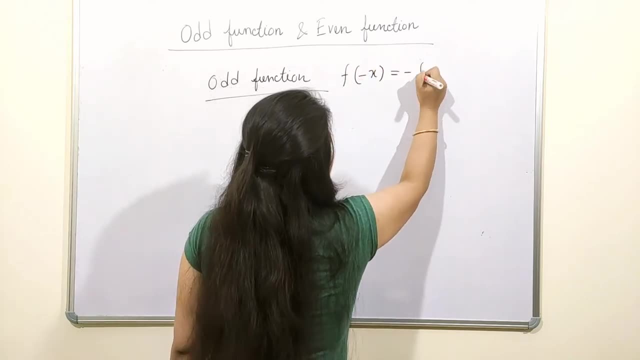 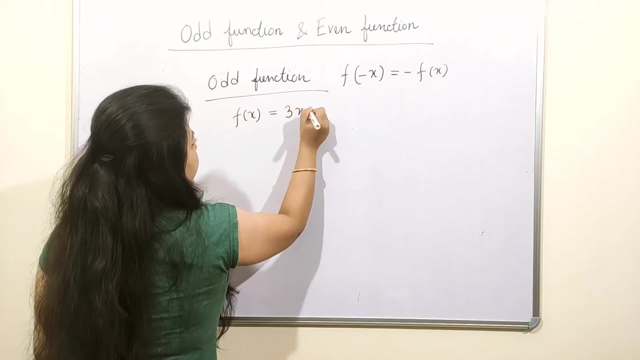 now let us discuss about the odd function. so f function will be called odd function whenever it is satisfied by the condition f minus x, equal to minus fx. that means koi bhi function. suppose fx amal loko ko mil gaya 3x cube plus 1, toh isme amal log dekhenge ki whether ye odd. 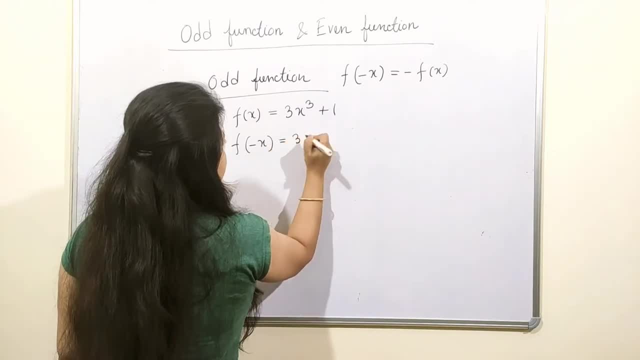 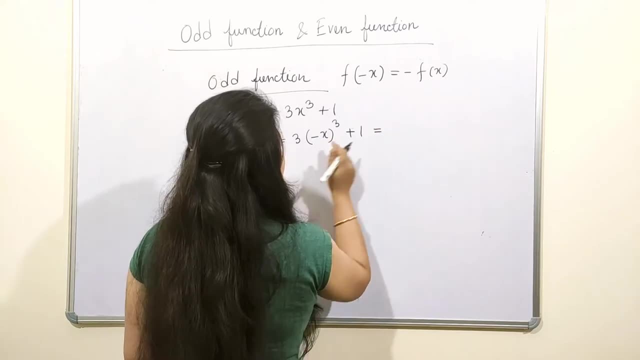 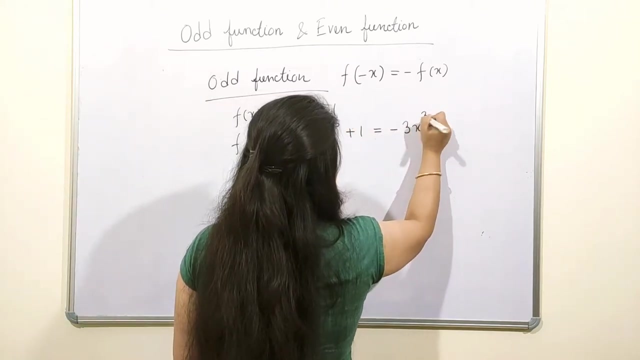 function hai ki nahi hai. so f minus x agar ho gaya. that means x ke place me amal loko replace. will be replaced by minus x cube plus 1, then what will be the value of minus x cube? minus x cube will also be there. so what we can write: 3 minus x cube plus 1. see what happened in this. 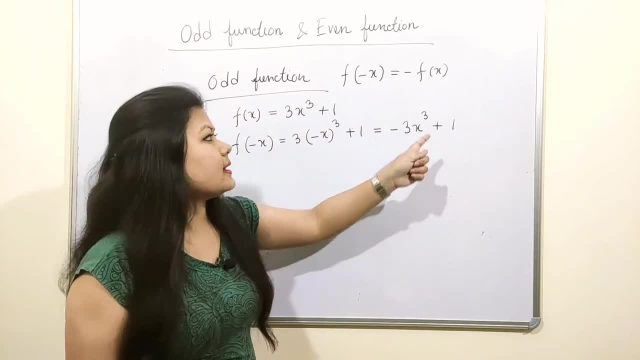 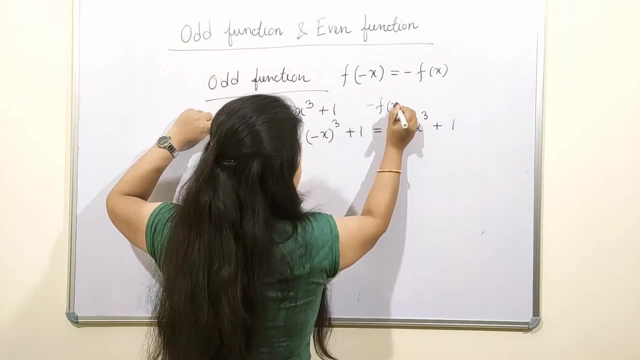 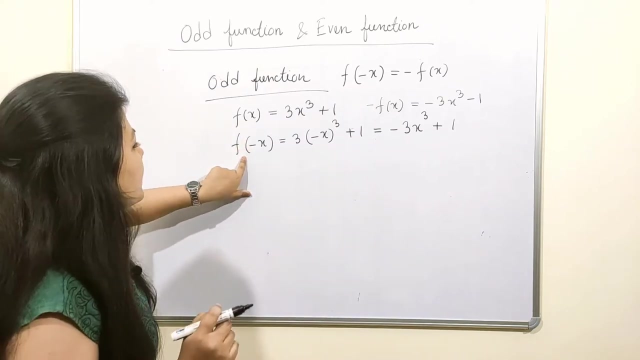 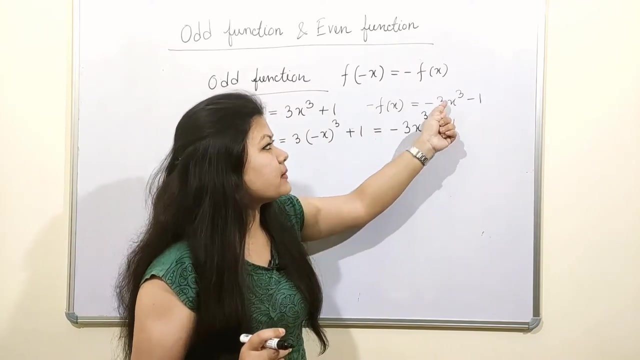 fx equal to. we got this value, but we did not get minus fx. if we directly multiply by minus, then we get minus 3x cube minus 1. but if we directly replace f minus x q, we got 3 minus 3 plus 1. that means this will also be minus 1 will be there. that's why this is not. 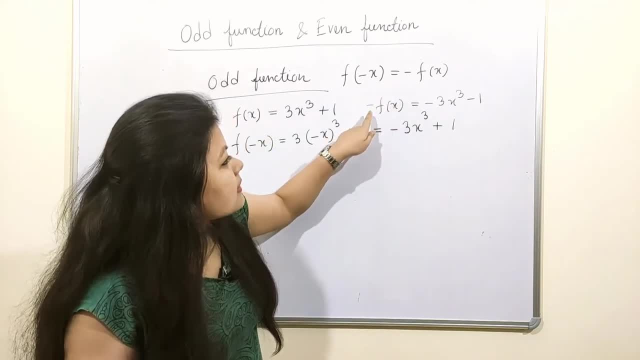 a odd function. remember what will happen in this: if this fx isár 분夠, if we multiply fx with minus, that fx will be flat. then minus 3x cube minus 1 will also be there. why will beavo come on? okay, and in this case, when we will see fx? simply, if we simply multiply it with minus,